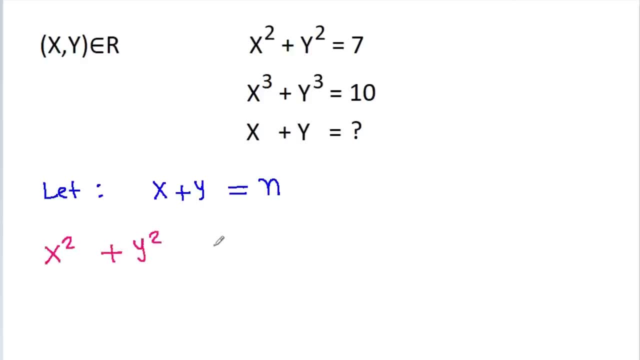 x square plus y square is equal to 7, and x square plus y square is equal to x plus y. whole square minus 2xy. that is equal to 7, and x plus y is equal to n, So it is n square minus 2xy is equal to 7, or we can get. 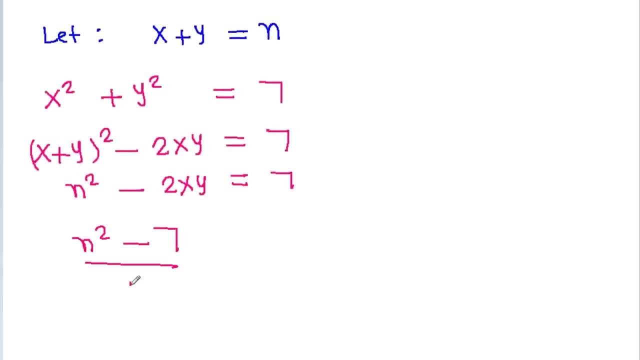 n square minus 7 by 2 is equal to xy. Suppose this is equation 1 and we have x cube plus y cube is equal to 10.. We have x cube plus y cube is equal to 10 and we know that a plus b whole cube is equal to a cube plus b. cube plus 3ab into a plus b. 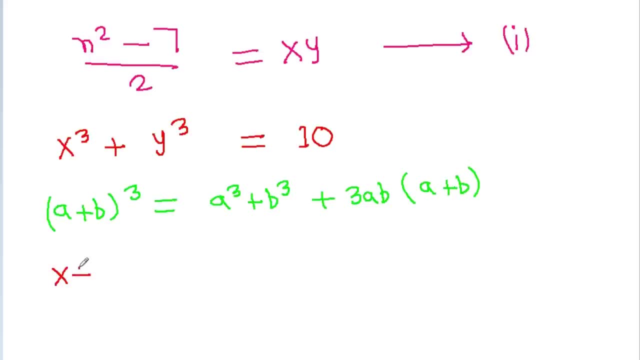 So x cube plus y cube will become x plus y, whole cube minus 3xy. x plus y, that is equal to 10 and x plus y is equal to n cube minus 3xy and x plus y is equal to n, is equal to 10 and we can get: nq minus 10 is equal to 3n. 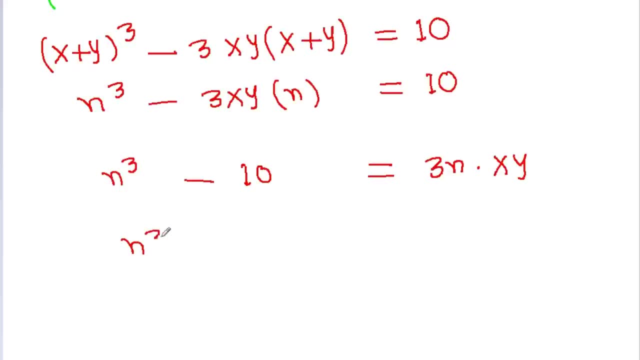 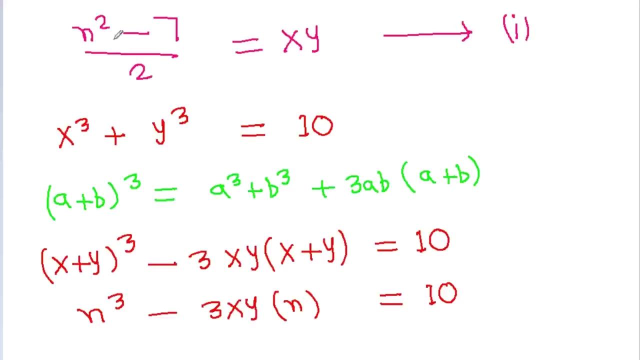 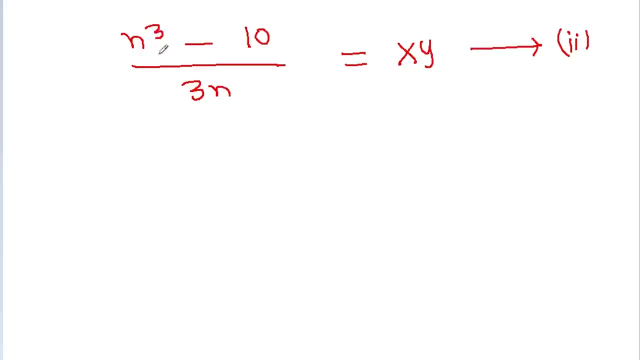 times xy, or nq minus 10 by 3n is equal to xy. Suppose this is equation 2 and now equation 1. it is xy is equal to n square minus 7 by 2, and equation 2 is xy is equal to nq minus 10 by 3n. So from equation 1 and equation 2 we can say: 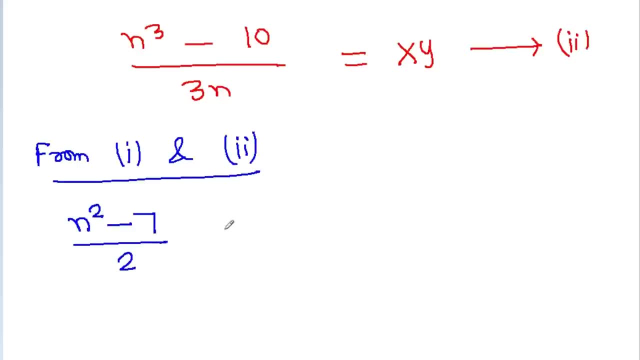 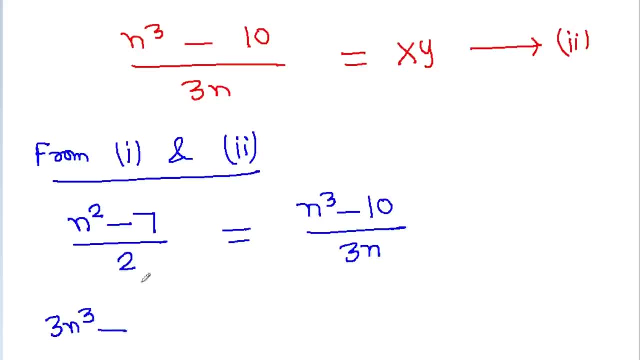 So from equation 1 and equation 2 we can say that n square minus 7 by 2 is equal to nq minus 10 by 3n, And it will be 3nq minus 7 into 3n will be 21n is equal to 2nq minus 20.. 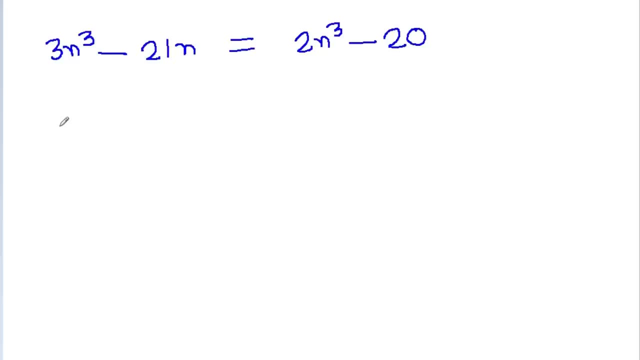 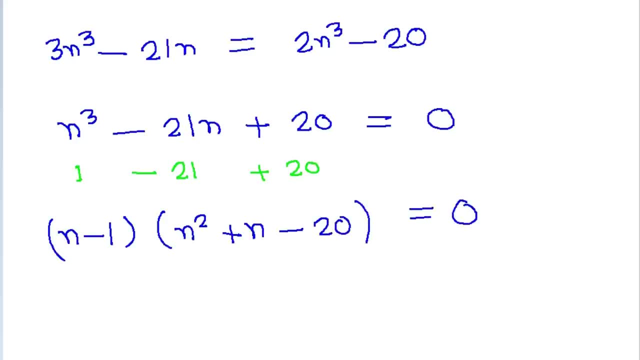 n is equal to 0. And now if we add 5 and minus 4, then we get 1.. And if we multiply 5 and minus 4, then we get minus 20.. So it will be n minus 1 times n plus 5 times n minus 4 is equal to 0. Or we can. 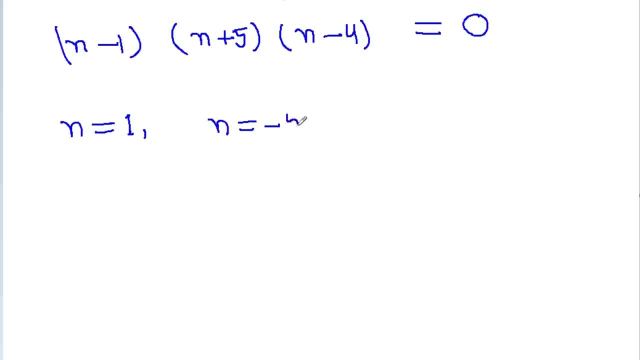 get n is equal to 1 and n is equal to minus 5 and n is equal to 4 and we have: x square plus y square is equal to 7 and x cube plus y cube is equal to 10 and x plus y is equal to n. We have x square plus y square is equal to 7 and x cube. 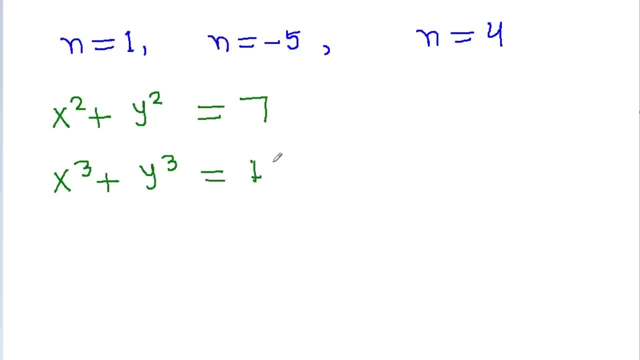 plus y cube is equal to 10, and x? y belongs to real numbers and we have: x plus y is equal to n, and n is equal to 4, and x plus y is also equal to minus 5, and x plus y is also equal to 1. and now 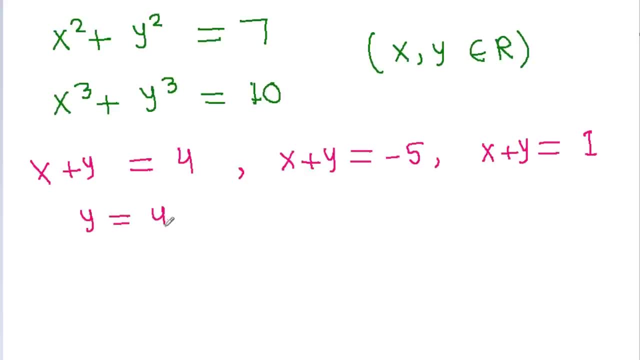 we can get: y is equal to 4 minus x, and here we can get: y is equal to minus 5 minus x, and here we can get: y is equal to 1 minus x, and we have: x square plus y. square is equal to 7. we have x square plus y. 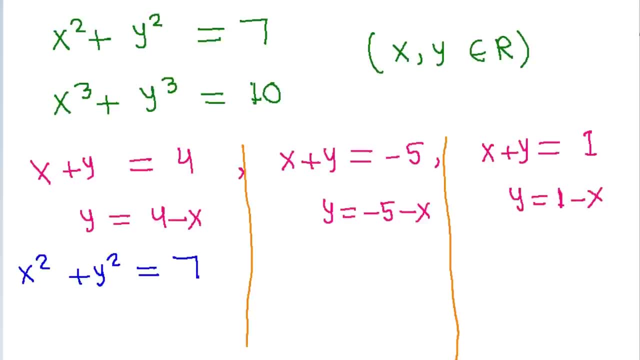 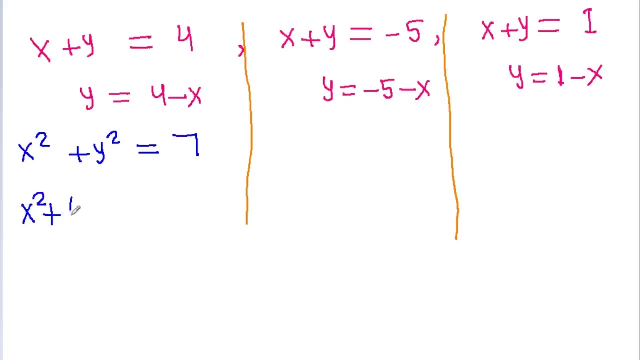 square is equal to 7, and it will be: x square plus y is equal to 4 minus x square is equal to 7, and it will be: x square plus 16 plus x square minus 8x is equal to 7, or 2x square minus 8x plus 16 minus 7 is 9 is equal to 0, and now 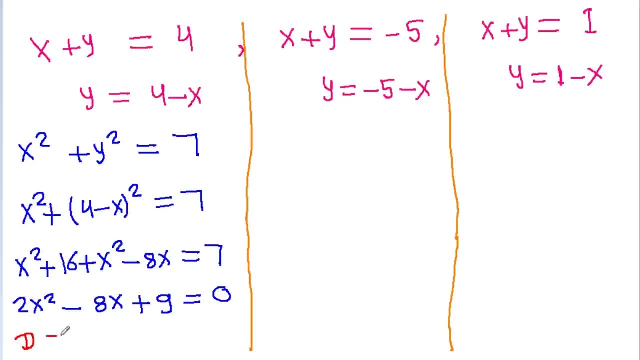 if we check discriminant. and now, if we check discriminant and now, if we check discriminant d, then it is equal to b square minus 4 d, then it is equal to b square minus 4 d, then it is equal to b square minus 4 ac, and b is minus 8 a square. 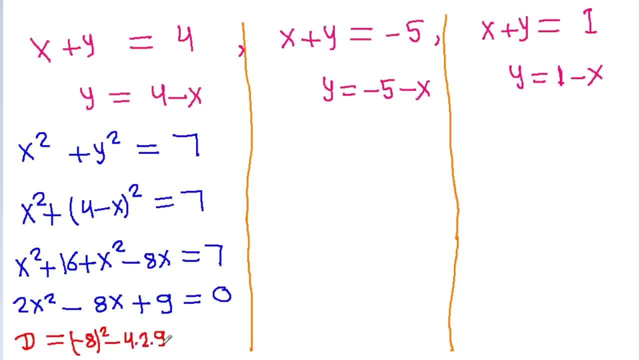 ac and b is minus 8. a square ac and b is minus 8. a square minus 4. into a is 2 and c is 9 minus 4 into a is 2 and c is 9 minus 4. into a is 2 and c is 9, and it will be 64 minus 72. 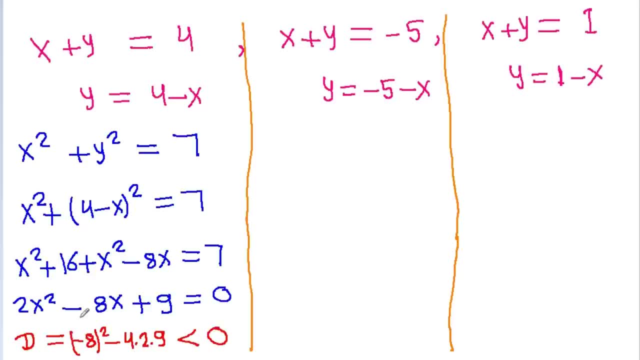 and it will be 64 minus 72, and it will be 64 minus 72. that is negative. so here we cannot get. that is negative. so here we cannot get. that is negative. so here we cannot get. real value of x, real value of x, real value of x. so x plus y cannot be equal to 4. 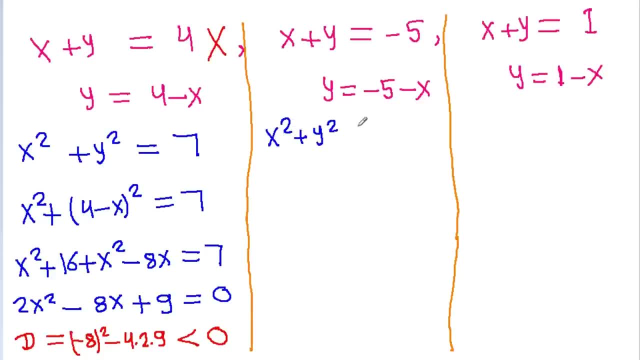 so x plus y cannot be equal to 4. so x plus y cannot be equal to 4. and here we have x square plus y square. and here we have x square plus y square is equal to 7, is equal to 7 is equal to 7, and x square plus y is equal to minus 5. 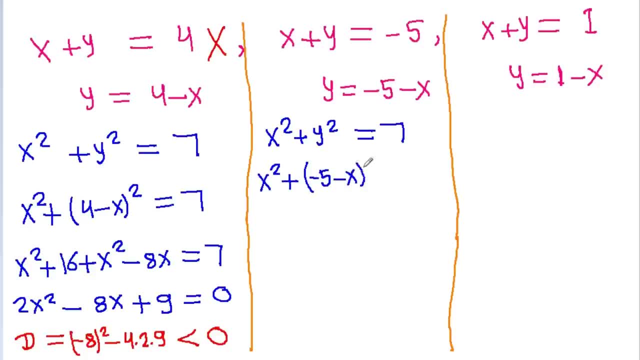 and x square plus y is equal to minus 5 and x square plus y is equal to minus 5 minus x. minus x minus x. y is minus 5 minus x. a square is equal to: y is minus 5 minus x. a square is equal to. 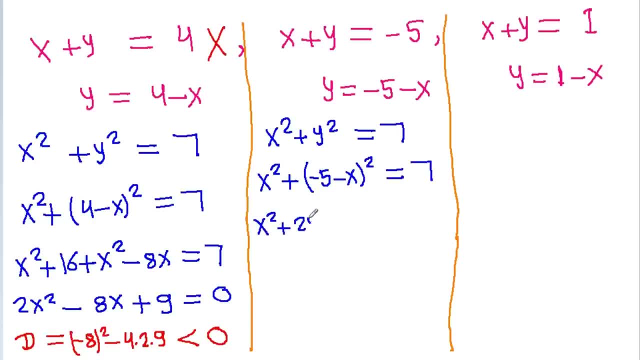 y is minus 5 minus x, a square is equal to 7, 7- 7, and it is x square plus 25, and it is x square plus 25, and it is x square plus 25 minus x square, minus x square minus x. square plus 10, x is equal to 7. 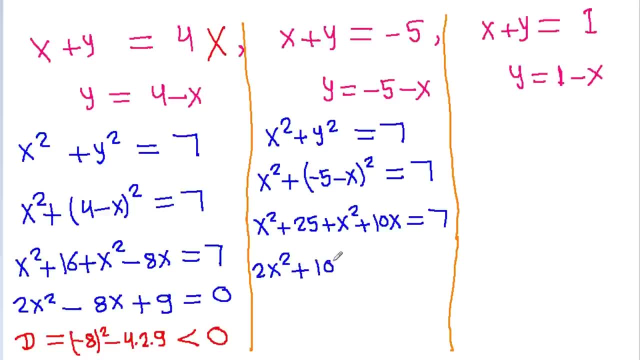 plus 10 x is equal to 7 plus 10 x is equal to 7, and we get 2 x square plus 10 x, and we get 2 x square plus 10 x, and we get 2 x square plus 10 x. plus 25 minus 7 is 18 is equal to 0. 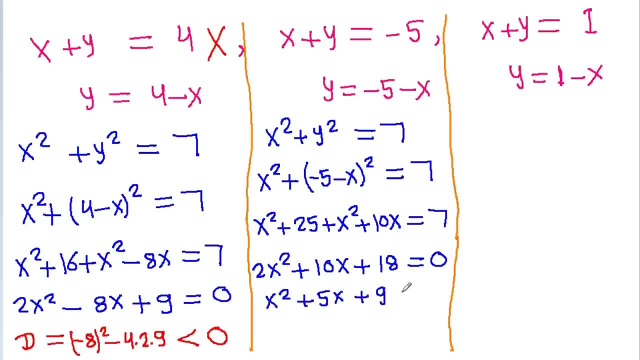 plus 25 minus 7 is equal to 0. plus 25 minus 7 is equal to 0, or x square plus 5 x, or x square plus 5 x, or x square plus 5 x plus 9 is equal to 0. 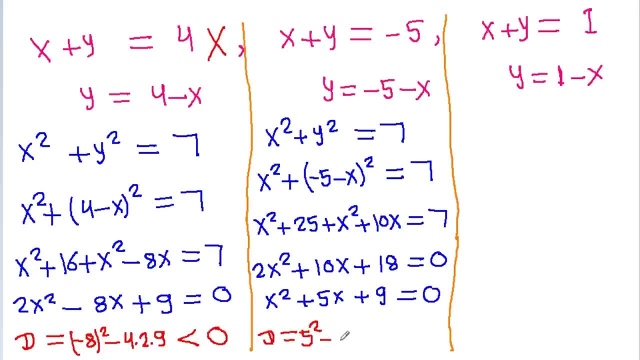 plus 9 is equal to 0 plus 9 is equal to 0, and now d will be 5 square minus, and now d will be 5 square minus, and now d will be 5 square minus 4 into 1, into 9. 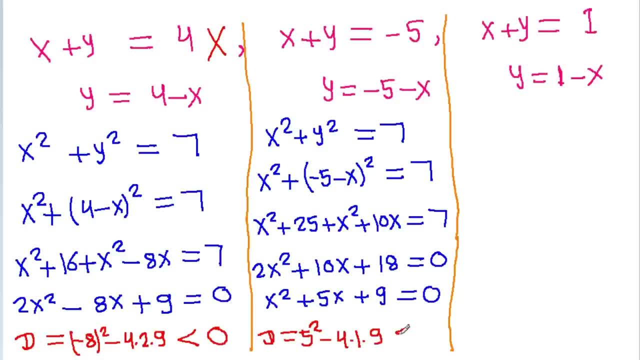 4 into 1 into 9. 4 into 1 into 9, that is 25 minus 36. that is 25 minus 36, that is 25 minus 36. so it is negative, so it is negative, so it is negative. so here also we cannot get real value. 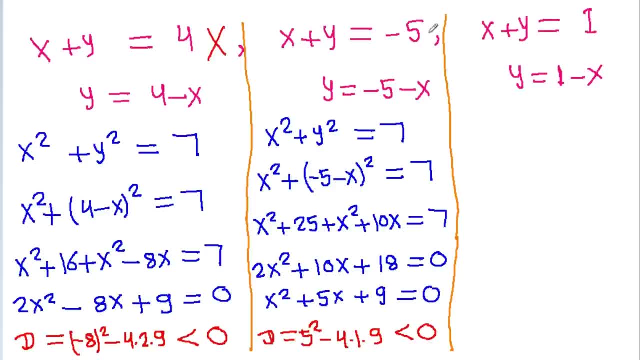 so here also we cannot get real value. so here also we cannot get real value of x, of x, of x. so x plus y also cannot be equal to. so x plus y also cannot be equal to. so x plus y also cannot be equal to minus 5. 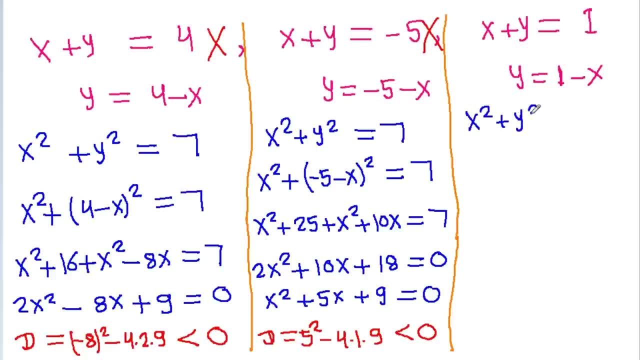 minus 5 minus 5, and here also we have x square plus y, and here also we have x square plus y, and here also we have x square plus y. square is equal to 7, square is equal to 7, square is equal to 7, and x square plus y is equal to 1 minus. 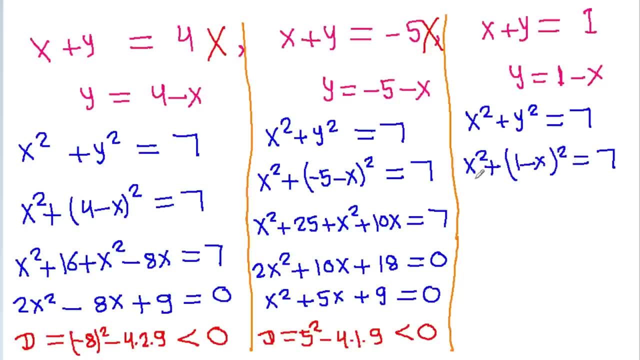 and x square plus y is equal to 1 minus and x square plus y is equal to 1 minus x. x. x square is equal to 7 and it is x square. square is equal to 7 and it is x square square is equal to 7 and it is x square minus: 1 minus x square. 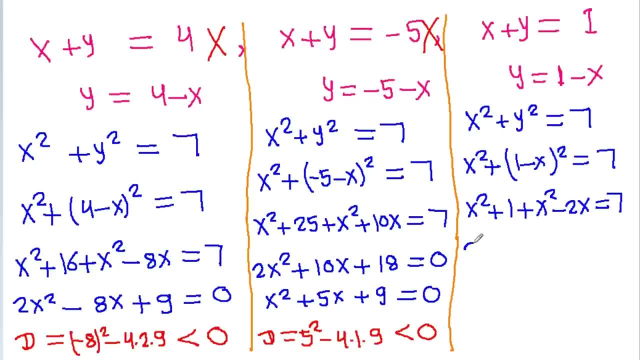 minus 1 minus x square minus 1 minus x. square minus 2 x is equal to 7 minus 2 x is equal to 7, and we get 2 x square and we get 2 x square and we get 2 x square minus 2 x and 1 minus 7. 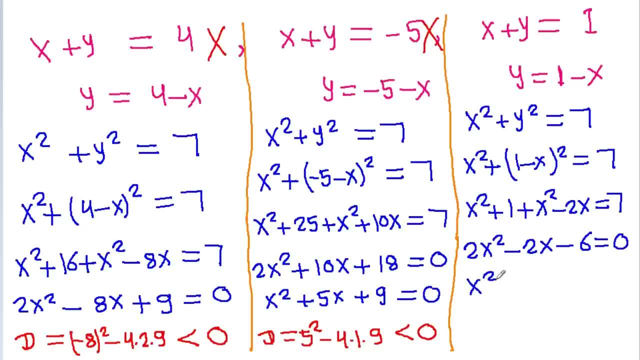 minus 2 x and 1 minus 7. minus 2 x and 1 minus 7 will be minus 6 is equal to 0 and x square minus x minus 3 and x square minus x minus 3 and x square minus x minus 3 is equal to 0, and.